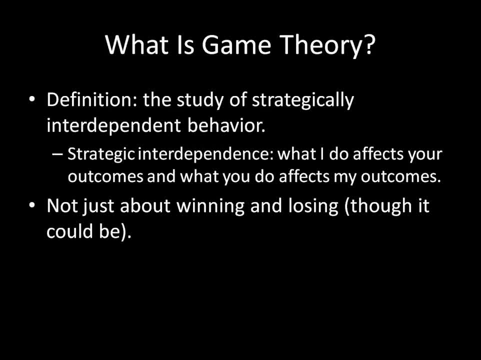 what game theory is? Game theory is simply the study of strategically interdependent behavior. Strategic interdependence is simply a way of describing situations where what I do affects your outcomes and what you do affects my outcomes. These types of situations could be just about winning and losing. I know when we think of the word game immediately. 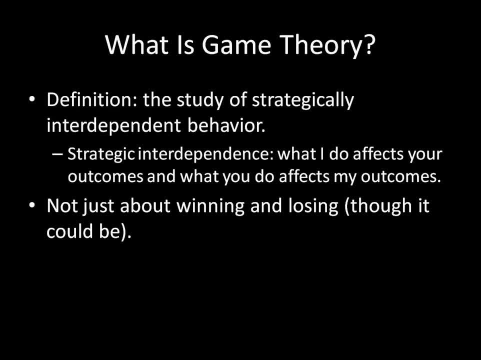 we think about types of games where I'm trying to beat you and you're trying to beat me, and only one of us can win and only one of us can lose. But game theory allows us to be a little bit more broad with what we're doing here. Our framework can be much more general. 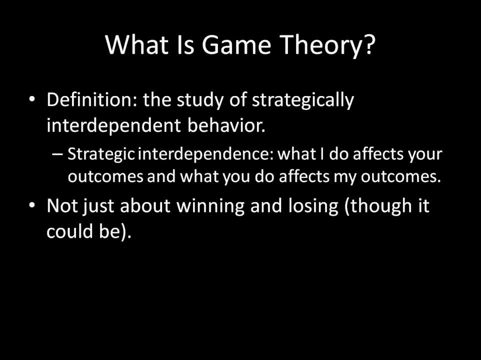 than that, and so we can talk about situations where we're both trying to help each other win, and also situations that are somewhere in between, where we have incentives to work together but also incentives to beat the other guy in some sense, And game theory is: 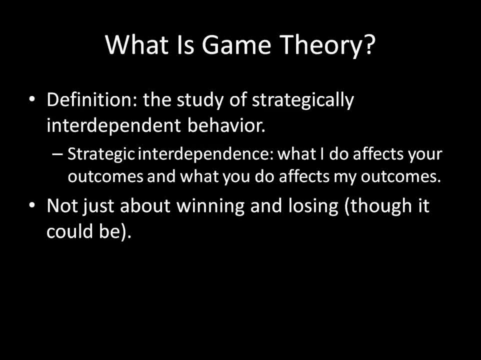 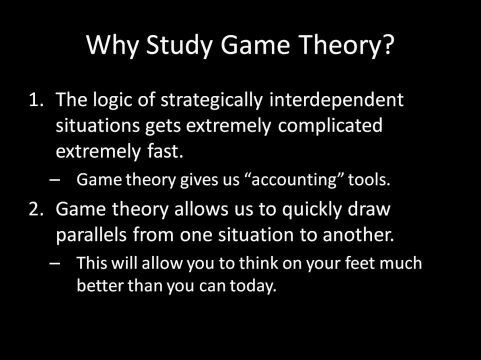 going to allow us to study that all in a single way. It's really useful. And to allude to what I'm going to talk about next, why even bother with these 30 to 40 videos? Because game theory will be time consuming. It's going to be logically. 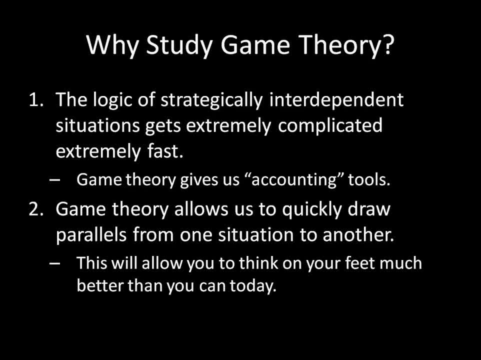 demanding for us to learn, but there is a light at the end of the tunnel. There is a reason, actually, I'm giving you two reasons- why we should bother doing this. First, if we're talking about theories of interactive behavior, the logic of strategically interdependent, 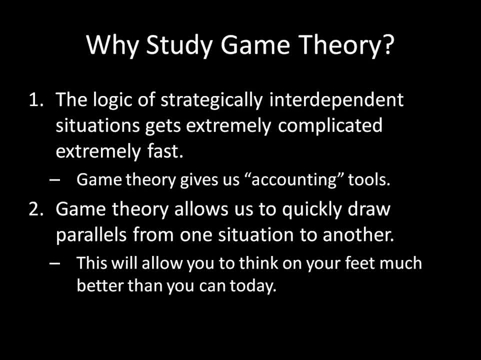 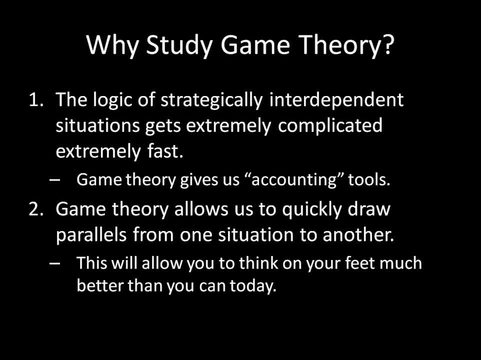 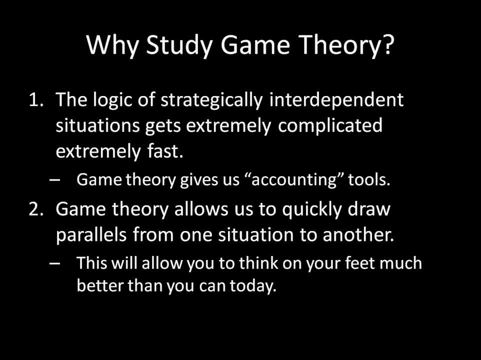 lecture series where I was in trouble with the police and my knowledge of game theory allowed me to get out of that situation with very little cost to myself. So we'll talk about that and why it was really useful to me once we get there. 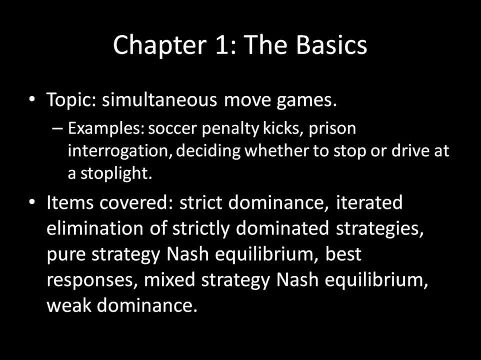 This lecture series will cover three chapters in total. We're going to start out with the basics, So in chapter one we're going to be talking about simultaneous move games. These are games where the players essentially have to come up with their strategies and 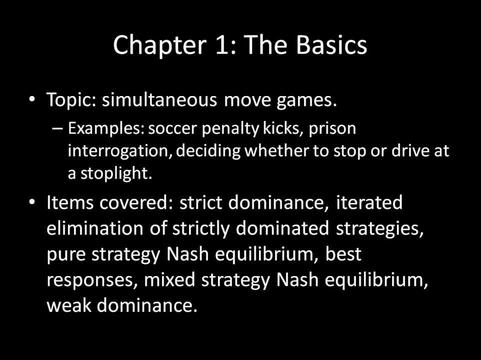 addressing them as they go along, Though I think that wouldn't happen without having independently and without observing what the other guy does. So some examples here include soccer penalty kicks, prison interrogation when you're isolated from your fellow criminals, and deciding whether to stop or drive at a stoplight. Now, over the course of this chapter, 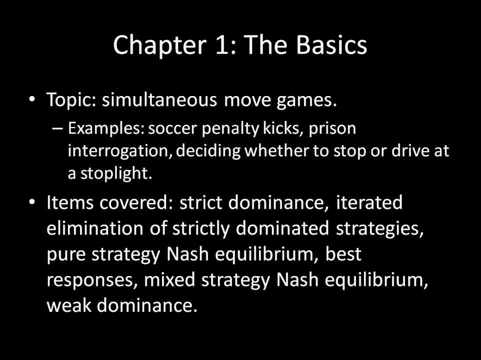 if you're interested in seeing what we're actually going to cover. we're going to talk about strict dominance, iterated elimination of strictly dominated strategies, peer strategy, Nash equilibrium, best responses, mixed strategy, Nash equilibrium and weak dominance. I don't 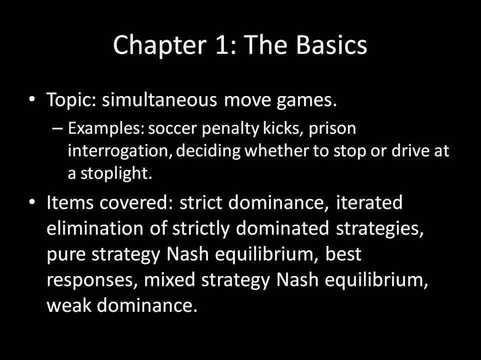 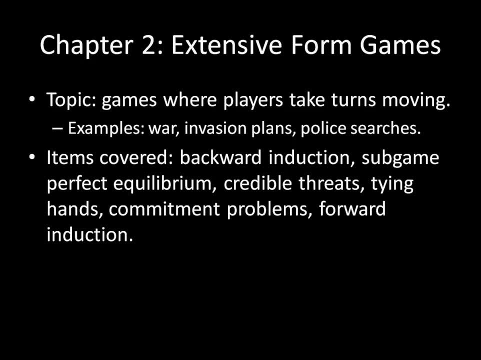 expect you to know any of those things yet, but by the end of chapter one you'll have those things down. I trust that Now in chapter two, we're going to move on to what we call extensive forum games, and this is the opposite of what we were doing earlier, before everyone was making 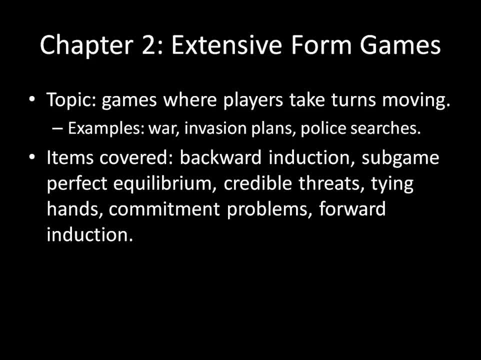 their moves at the same time. Here the players are taking turns moving. So some examples here are war and invasion plans and police searches. That's getting to what I was talking about before, where I have to decide whether to allow the police officer to search and then, once I have 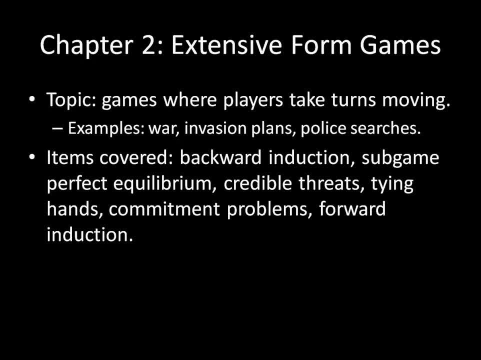 allowed the police officer to do that. then he decides whether to conduct a really thorough search or a really simple search. So these are times where you're going to have to make sure that you're doing the right thing, Just when we're taking turns moving And the items we'll cover in this chapter are backward. 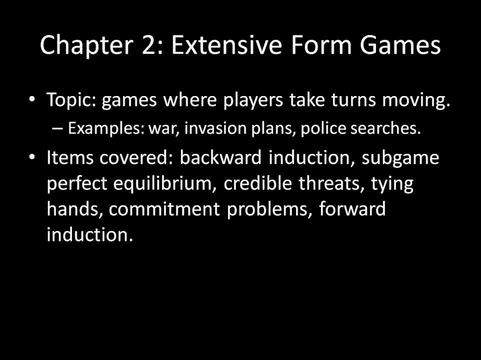 induction sub-game: perfect equilibrium, credible threats, tying hands, commitment problems and forward induction. Again, I don't expect you to know any of that coming into this, but by the end of chapter two you will have those things down. Now, the last chapter, we'll talk. 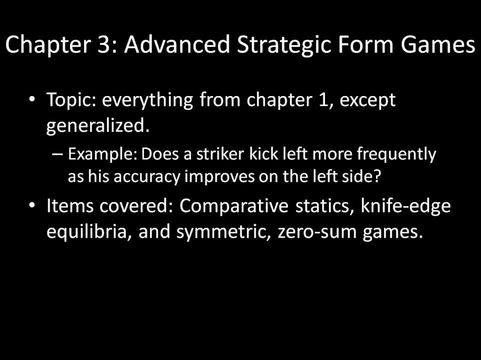 about advanced strategic forum games. So this is essentially what we covered in chapter one, except we're going to generalize it. So this allows us to ask really important questions like: does a striker kick left more frequently when he's kicking a penalty kick in soccer, As is? 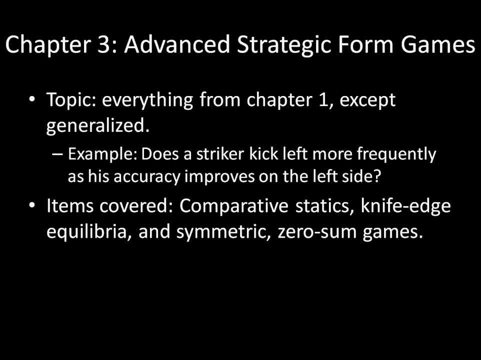 accuracy to the left side improves, And in this chapter, we'll be talking about comparative statics, which is really the heart and soul of game theory: knife edge equilibria and symmetric zero-sum games. Now, in terms of practical parts of this course, what are the prerequisites? Well, 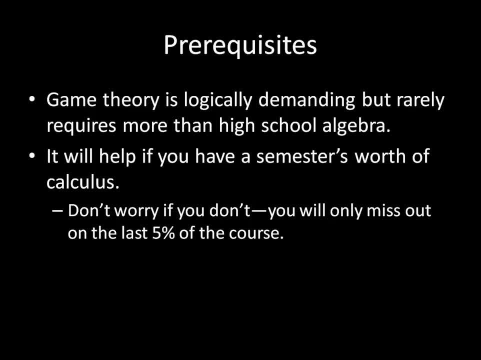 game theory is logically demanding but rarely requires more than high school algebra. It will help you if you have had a semester's worth of calculus, but even if you haven't, you'll only miss out on what's essentially the last 5% of the course. So even if you have tiny, tiny, tiny, 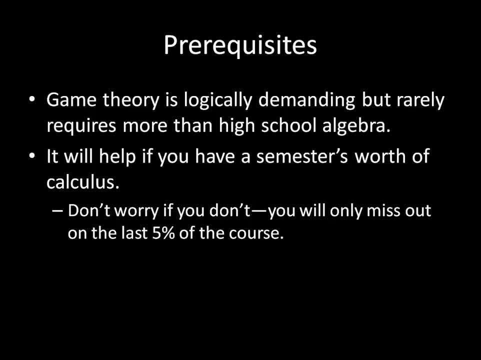 amounts of math, you'll still be able to get the most out of it. So if you have a semester's worth of calculus, you'll still be able to do this. Me personally: I got B's and C's in my high school. 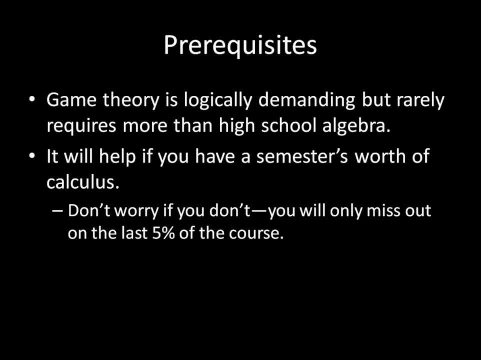 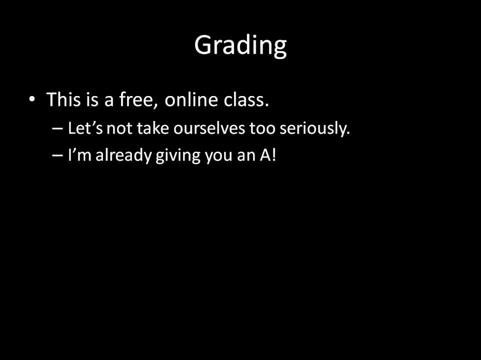 math classes, and now I do this. So if I'm capable of doing this, I think you're probably capable of doing this, as long as you put in the time and effort to really think about these things. Now grading: This is an online class. Let's not take ourselves so seriously. 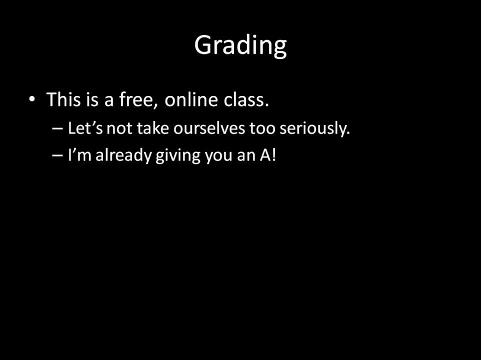 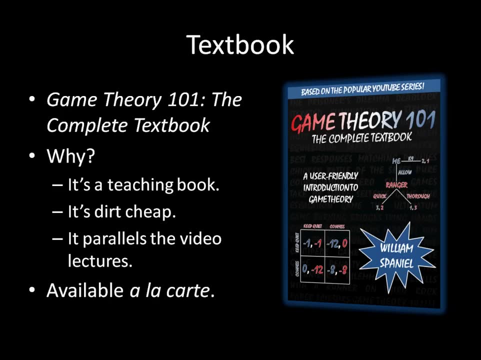 Congratulations: by watching this video, and this video only, You've already got an A in the course. Good job. Let's never talk about grades again, because that's ridiculous. Finally, in terms of a textbook, again, this is an online class. There are no required textbooks. 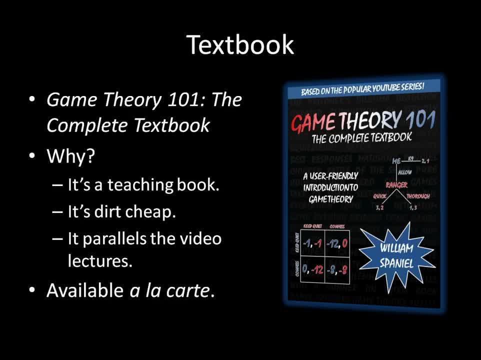 because this is just a made-up thing where you've already gotten an A. But that aside, if you are interested in looking into getting a textbook, this is what I recommend. It's Game Theory 101, the complete textbook. There's an obvious reason why I'm recommending it to you. 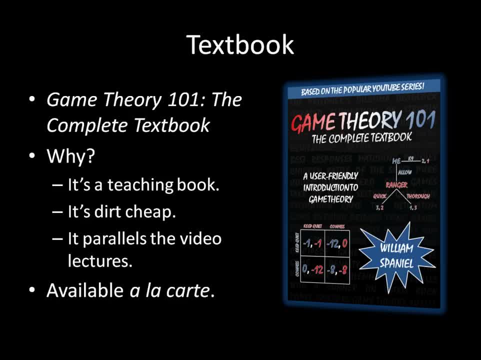 It's because I wrote it, But the reason I wrote it is so I could parallel the video series that I'm doing here, And so what we'll be doing in these lectures actually comes directly out of the book. But the book has many, many, many more examples in every lesson, whereas the video series 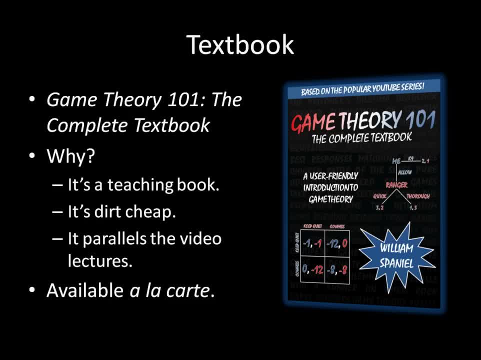 will just have one per lesson, So it parallels the video lectures very nicely. It's also dirt cheap As I film this: it's $3.99 on Amazon, So that's going to be way cheaper than any other options out there. And then finally, for practical reasons, it's also a teaching book. If you look at.